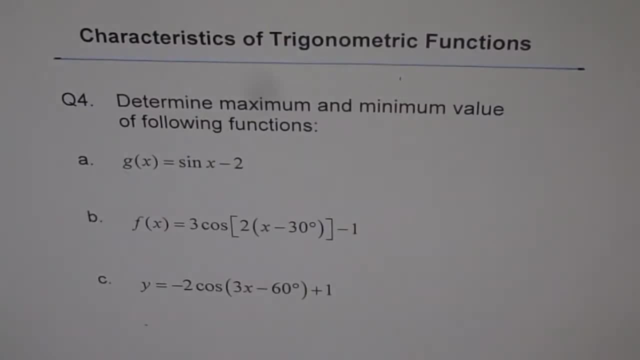 Characteristics of trigonometric functions. Question 4. Determine maximum and minimum value of the following functions. We have: g of x equals to sine x minus 2 as a and b is f of x equals to 3 cos of 2 times x minus 30 degrees minus 1. and c is y equals to minus 2 cos of 3x. 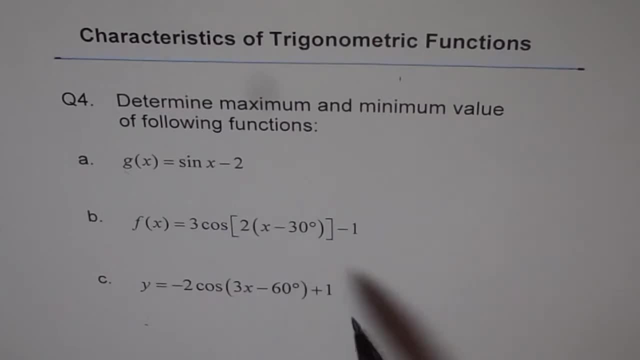 minus 60 degrees plus 1.. So in these three equations we find that all of them have been translated up and down, and so when there is a vertical translation, the maximum and minimum value changes. Maximum and minimum value also changes with vertical stretch or compression. 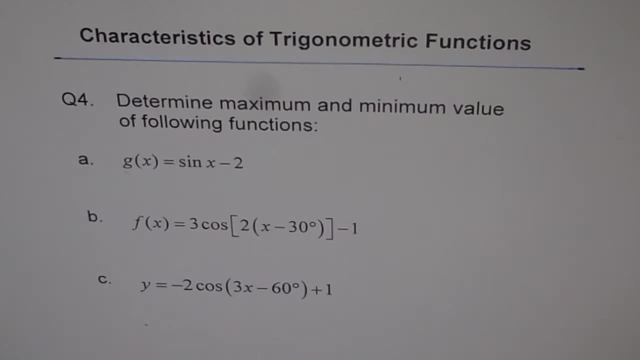 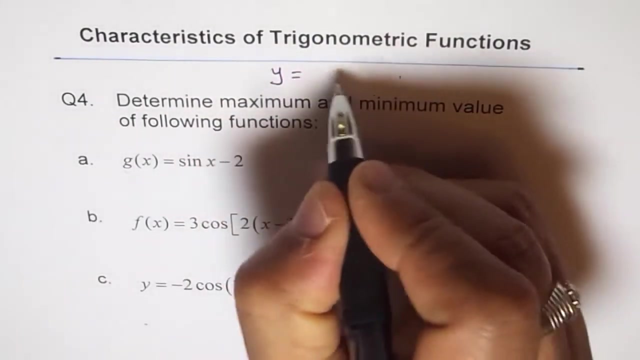 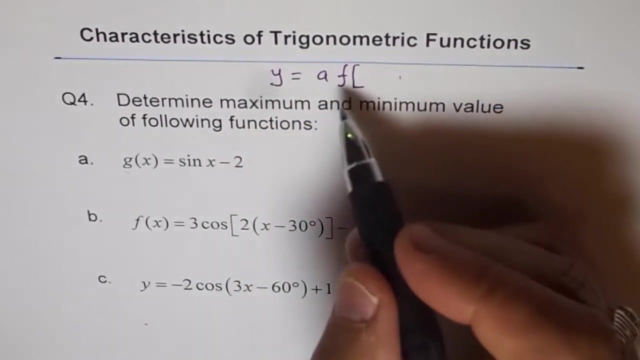 So basically, in any equation, in any trigonometric equation, the maximum and minimum value changes. The maximum and minimum value change is affected by vertical translation, whether it is vertical stretch or vertical translation. So in general, we will write a transformed equation like this can be written as: y equals to. let me write this a times f of, so it may be function. 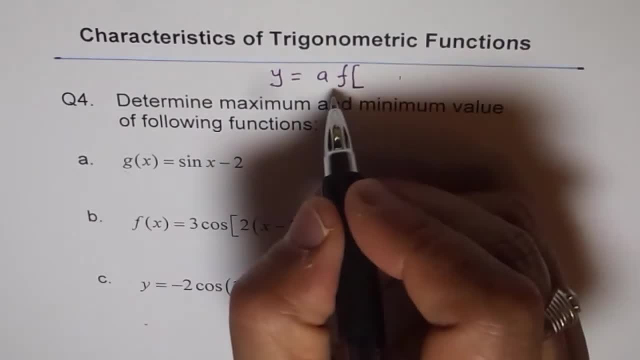 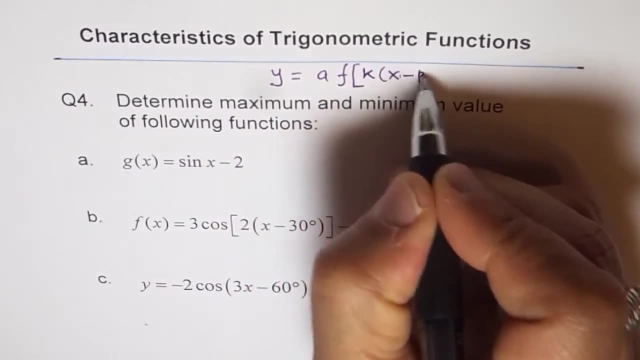 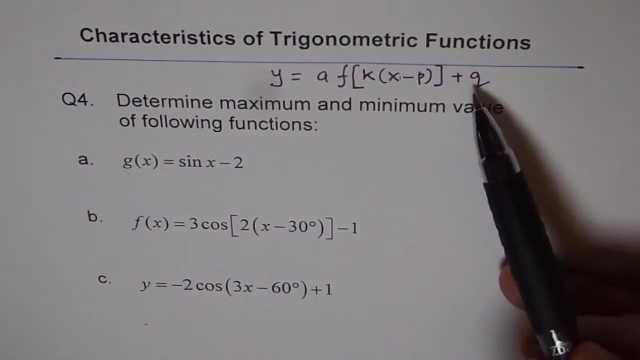 could be sine or cosine, and therefore we are writing f here. It could be sine, cosine or f of So it may be. function could be sine or cosine, and therefore we are writing f here. any function, k times x minus p plus q. right Books sometimes will write d here and c here. 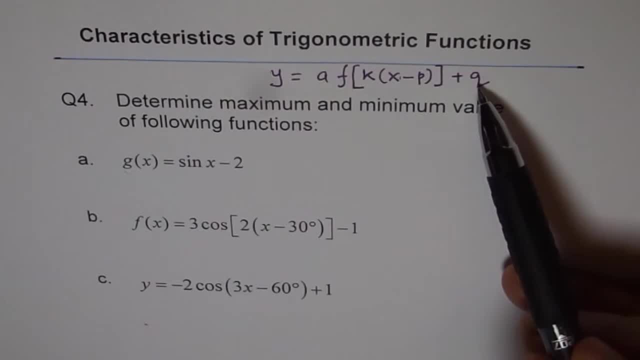 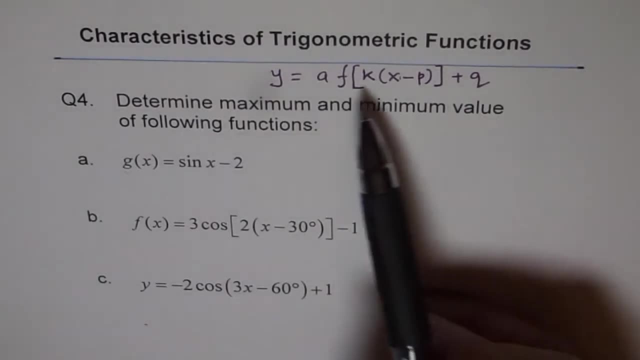 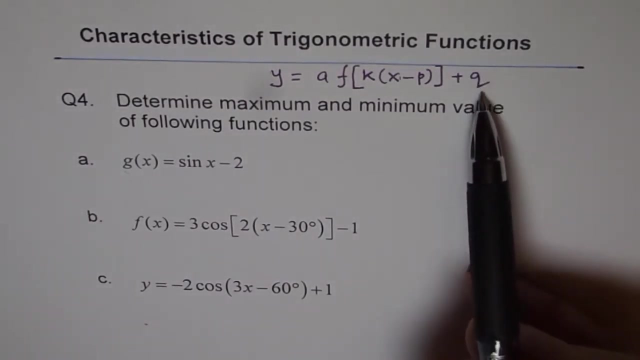 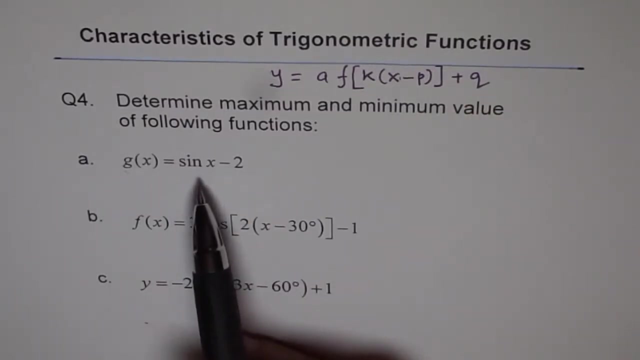 so p- I'm writing for phase shift right, And q is a vertical translation. So in this transformed equation or a general equation for a function, a represents a vertical stretch or compression and q represents the translation, vertical translation. correct Now for a sinusoidal function, whether it is a sine function or a cosine function, your. 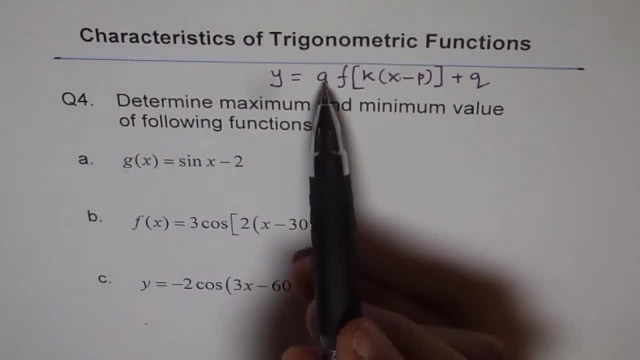 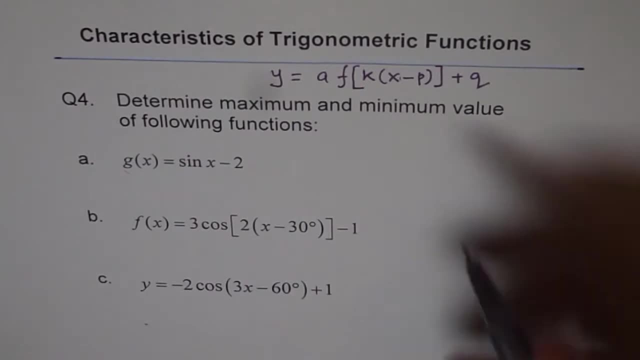 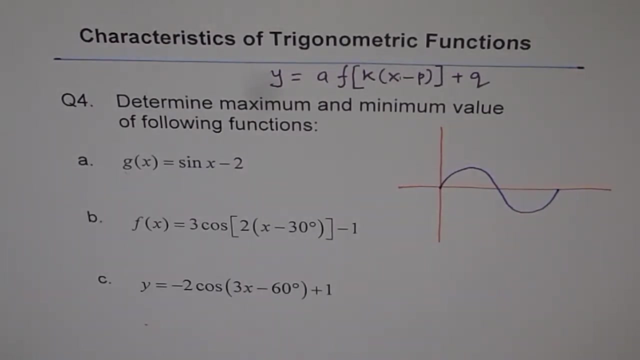 maximum and minimum values will be a plus q right. Why it is so? Let's try to understand that part. Okay, so here is my axis and let me draw a sine wave here. We'll just draw one sine wave to understand the concept. Now, if this is the wave, then 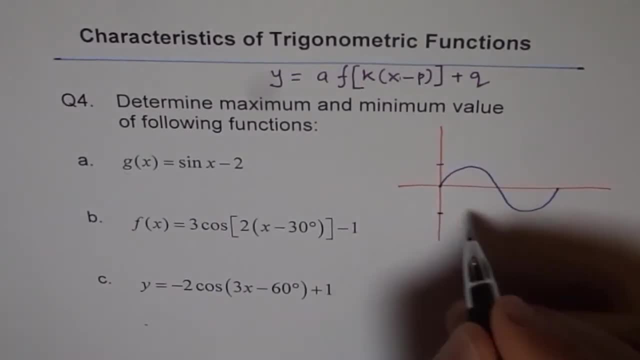 the amplitude is. let us say: amplitude is something a plus, this point is a and this point is a minus. let us say: right, So it has been already vertically stretched or compressed, correct Now. so the amplitude is always taken positive, whether it is showing like this: 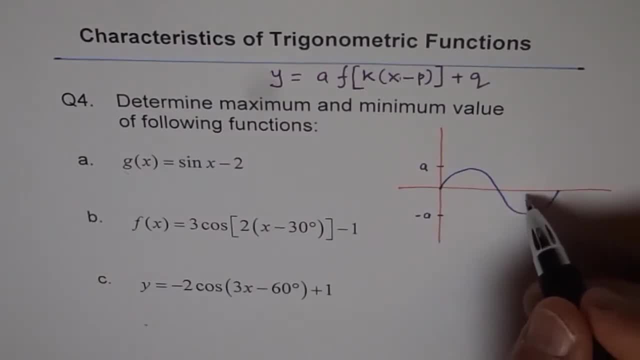 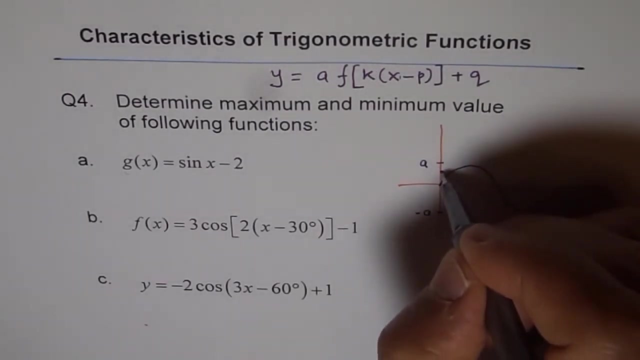 how a wave it goes from the mean value, which is axis of symmetry. The mean value is given by q, correct? Now if I transform this or translate it a bit, that means up and down. if I move this wave, let's say I move it at some position here, right, Let's say I make. 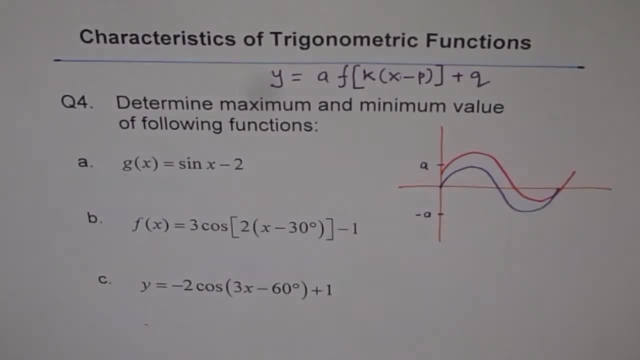 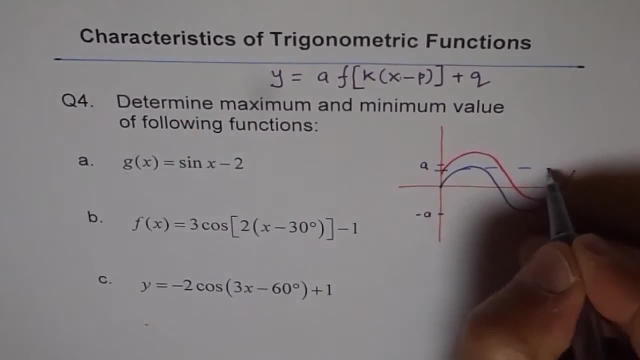 it like this, correct, And what I'm trying to say is that let me move it, let me move it right, And let's say this point becomes: this point becomes q- for me it is the units which I have- or let me separately draw it, that's better. So we'll compare it with this. 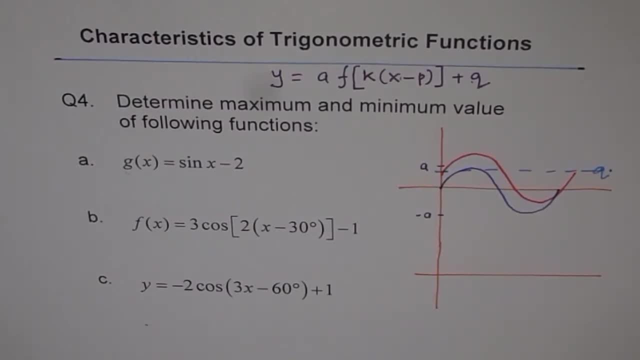 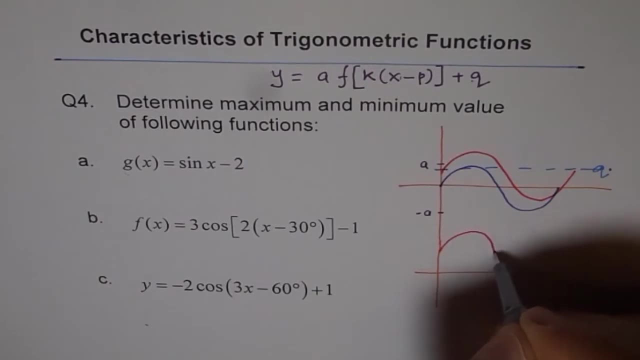 drawing correct. That will be good for us. So let's say, now we draw another wave, not here, but we draw it here. let's say this point: Okay, it could, it may or may not touch it, it doesn't really matter. 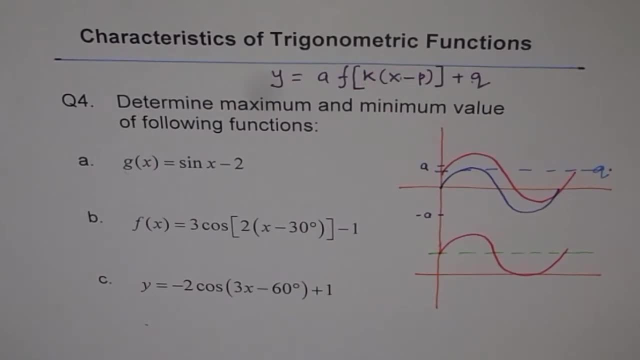 Let's say: this is our wave now. So where what I'm trying to say is: this is your vertical translation: q. let's say write q here, right, So that is q for us, And a is how far away you go from q in the positive side and negative side, Since this is axis of symmetry, both. 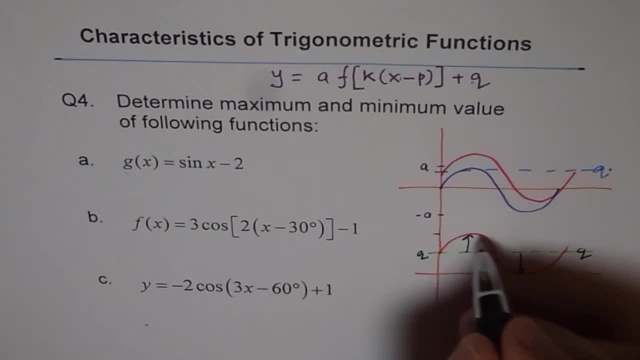 these distances are same, So this point will be what This point will be: q plus a right, q plus a And this point will be q minus a. Do you see that? So that is how you get your maximum and minimum. So, in finding maximum, 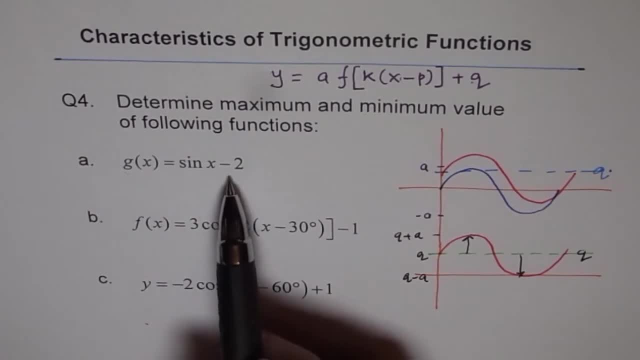 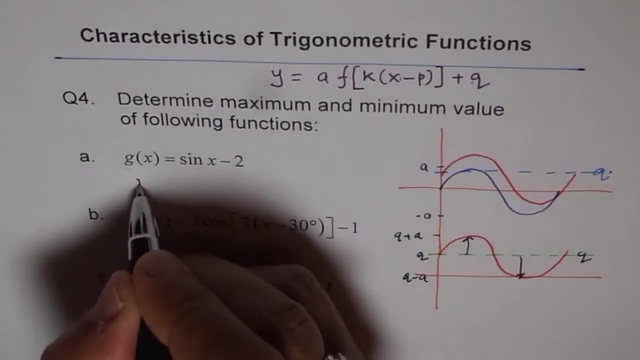 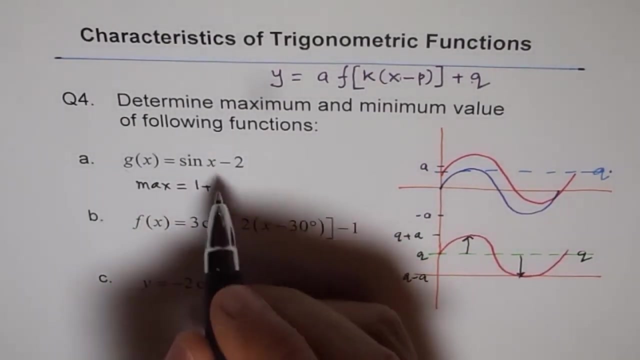 and minimum. what you have to do is you have to figure out what is the vertical translation and what is the vertical stretch at there to get your answer. So here it's easy. now We get: maximum is equal to a is 1 for us. So we get 1 plus q is minus 2.. So we'll do. 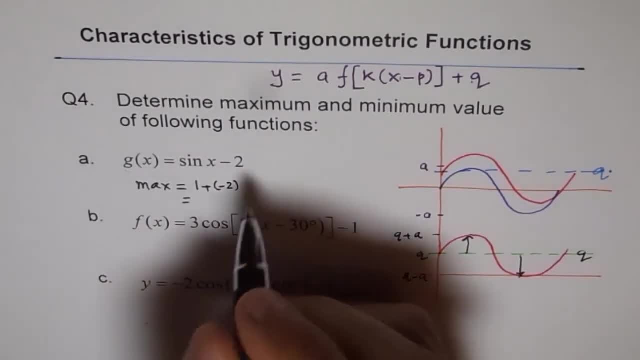 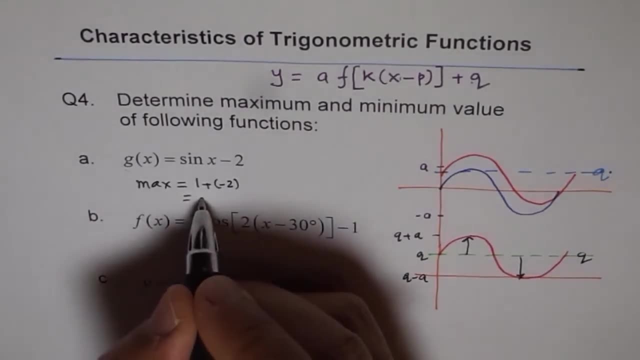 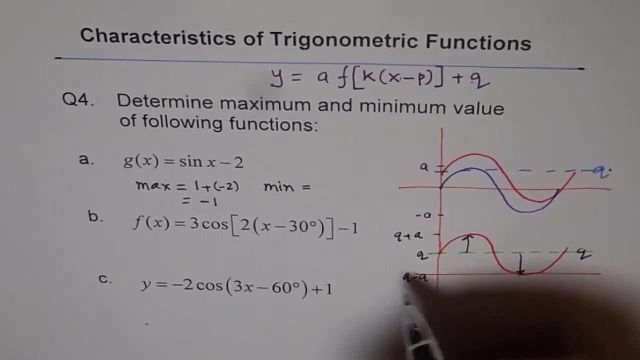 minus 2, correct, And therefore we get Yeah maximum position could be negative or positive. Remember that. So this is minus 1, correct And the minimum for us will be q minus a. q is we'll write q first now. 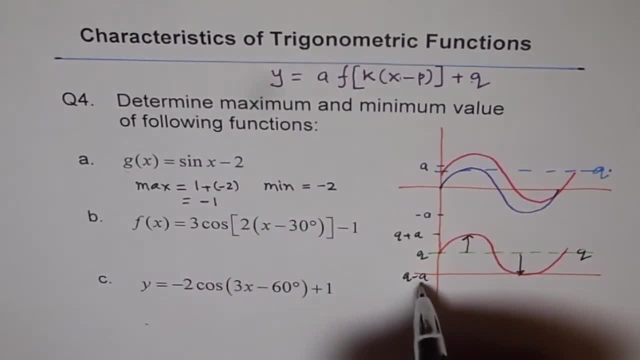 okay, q is minus 2.. Minus 2 and minus a, a is 1.. So it's minus 1.. So it will be minus 3, right? So this wave is is kind of kind of here, Do you see that Okay? 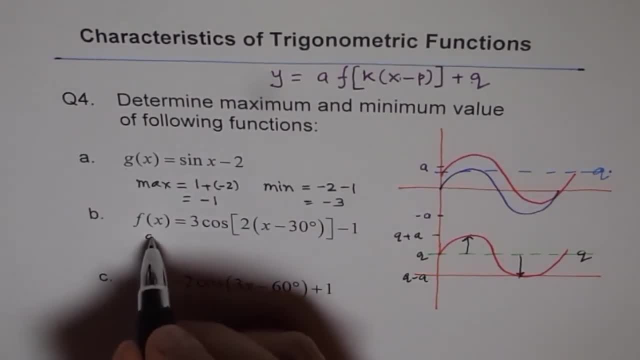 Now there for this function, what is a, a is 3 for us and q is minus 1.. And therefore our maximum will be: add them up. That is minus 1 plus 3, which is 2.. And minimum will. 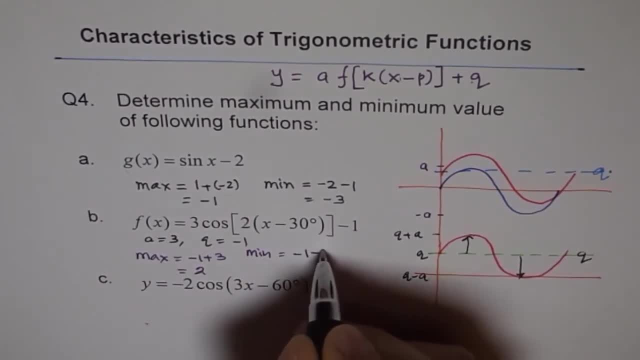 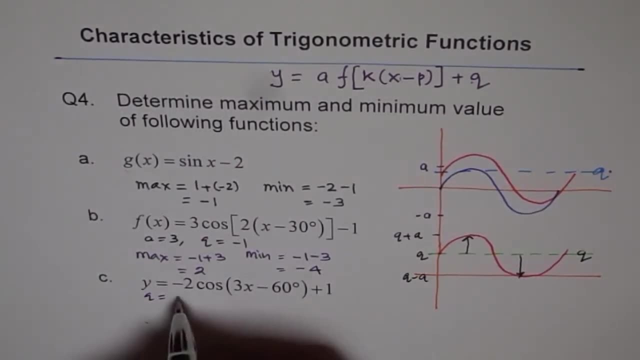 be minus 1 minus 3, which would be minus 4.. Perfect. Now, here we'll write q first. q equals to 1.. a equals to minus 2.. Maximum will be: you do it. And minimum will be: you do it, correct.